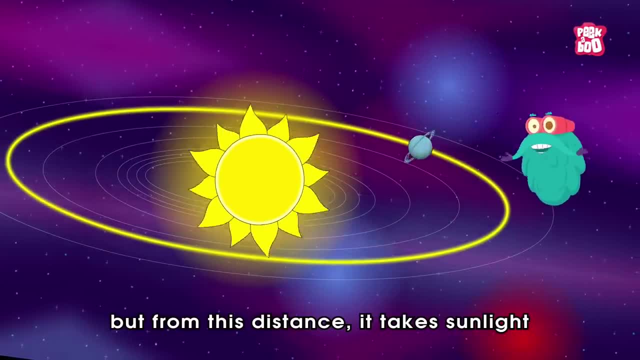 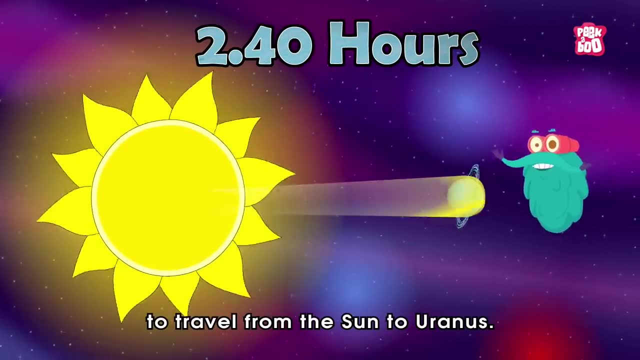 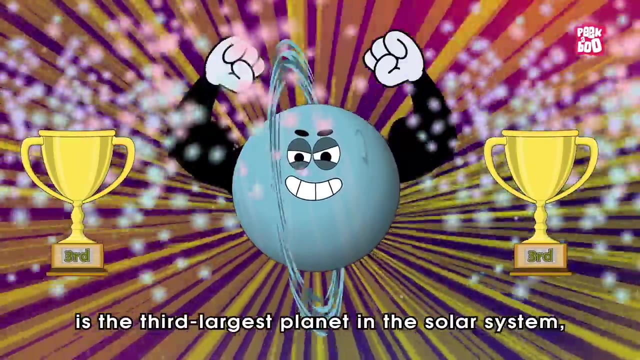 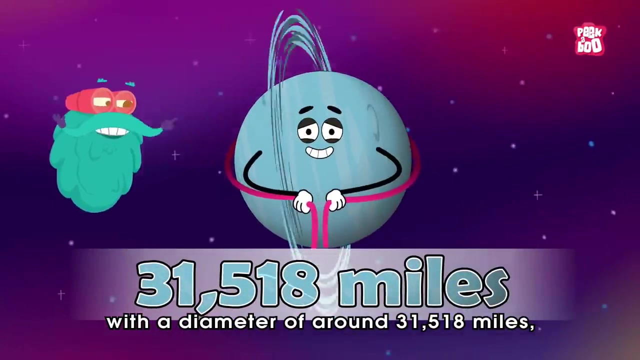 And you won't believe it, but from this distance, it takes sunlight 2 hours and 40 minutes to travel from the Sun to Uranus. But let's not forget that Uranus is the third largest planet in the Solar System, with a diameter of around 31,518 miles, which is about 4 times wider than Earth. 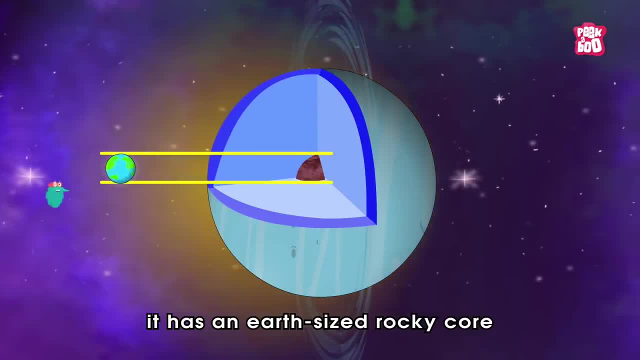 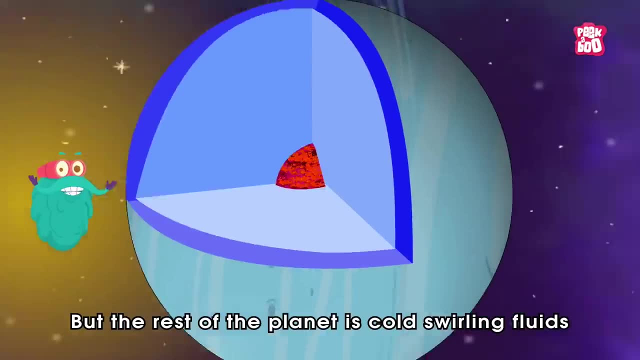 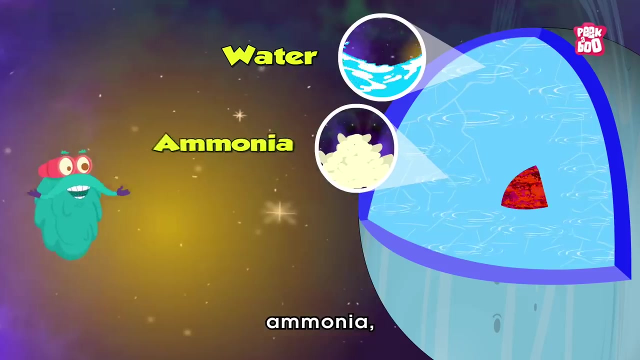 At the center it has an Earth-sized rocky core burning with a temperature of nearly 9,000 degrees Fahrenheit, But the rest of the planet is cold, swirling fluids consisting of water, ammonia and methane, which gives Uranus its iconic blue color. 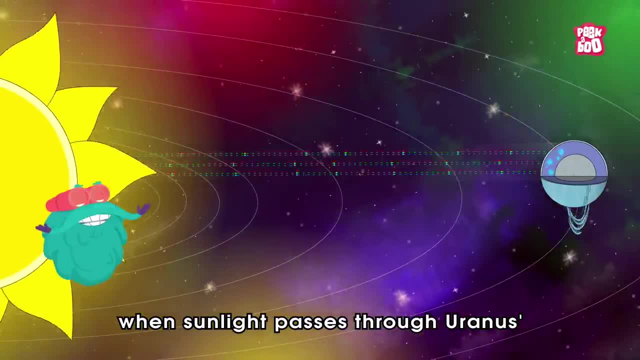 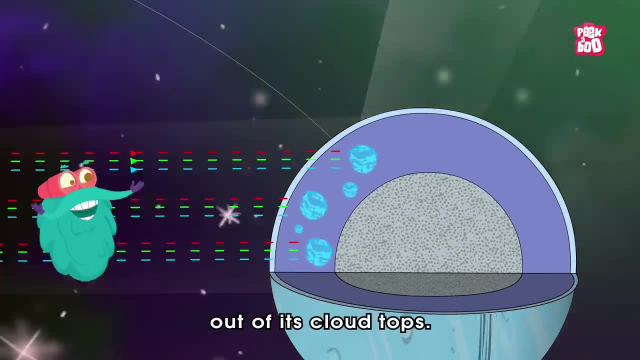 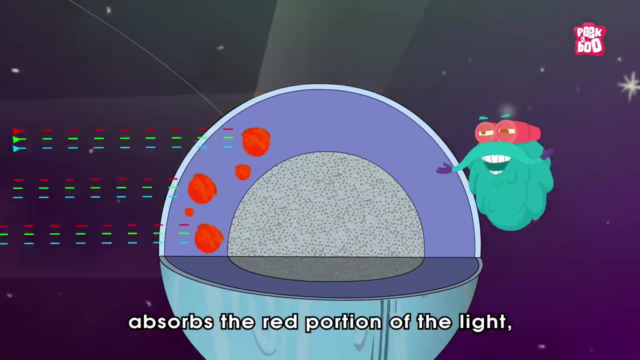 Yes, when sunlight passes through Uranus atmosphere made mostly of hydrogen and helium, the rays are reflected back out of its core, out of its cloud tops, and when that happens, the little methane gas present in it absorbs the red portion of the light. 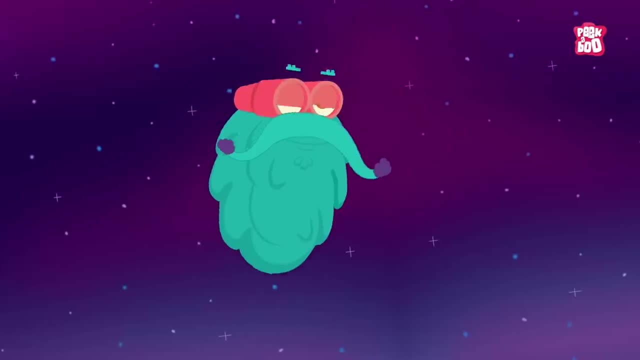 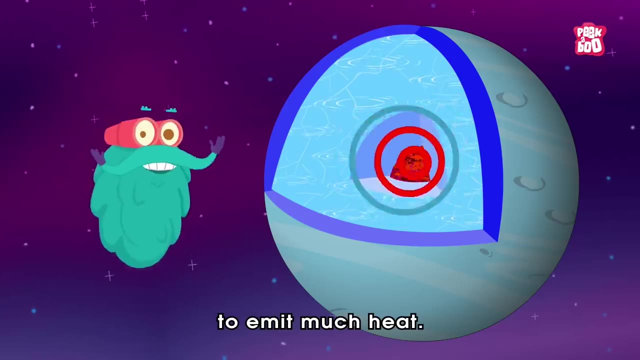 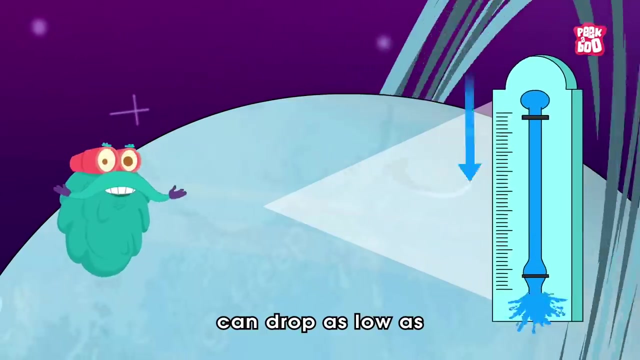 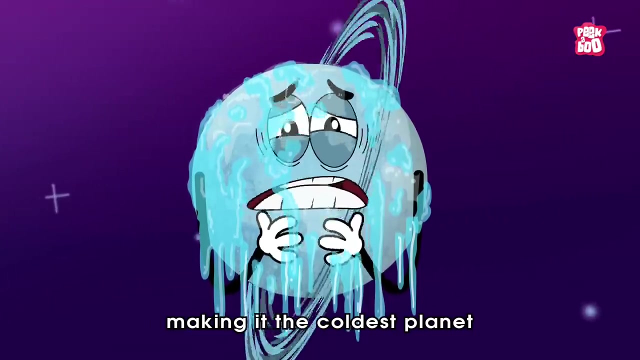 resulting in a blue-green color. Not only that, all this chemical composition does not allow Uranus to emit much heat. As a result, the temperature on its liquidy surface can drop as low as 70 degrees Fahrenheit, making it the coldest planet in our Solar System. 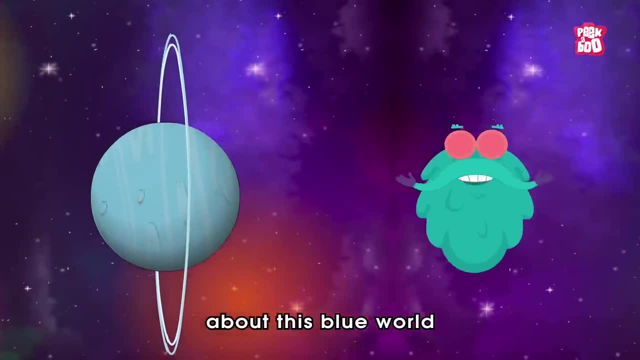 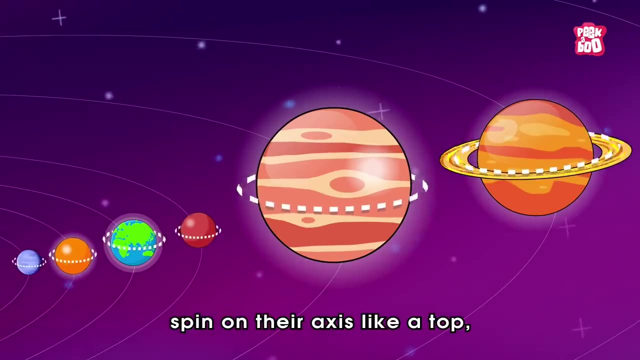 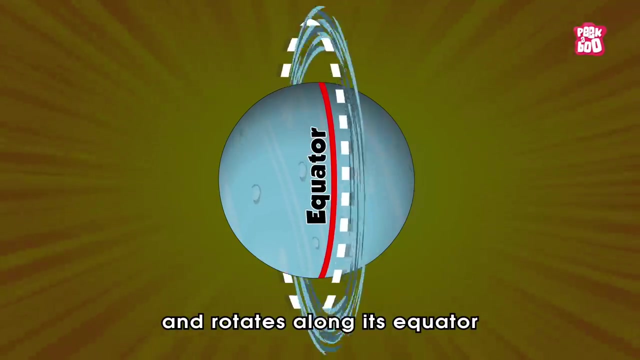 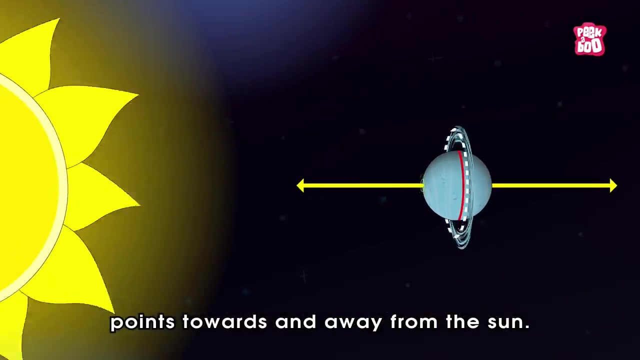 But the most fascinating thing about this blue world is its strange orientation. Yes, while the other seven planets spin on their axis like a top, Uranus takes a different turn and rotates along its equator at a right angle, in which its polar region points towards and away from the Sun. 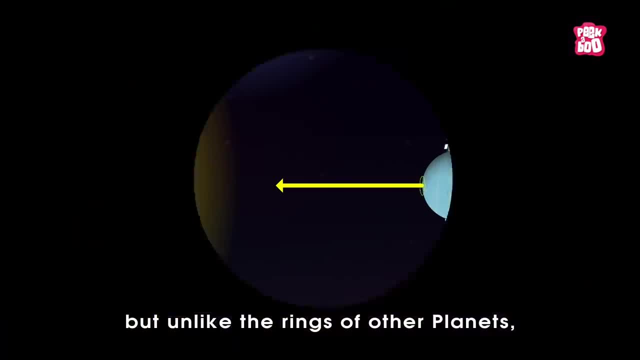 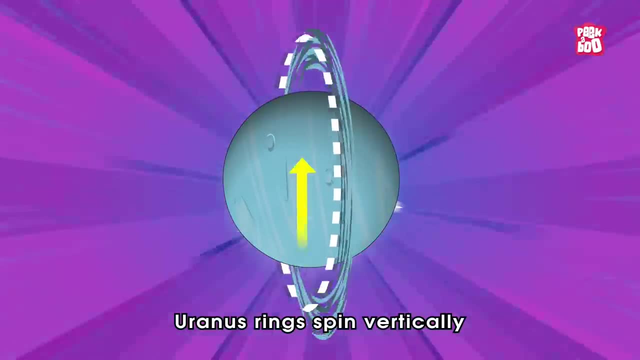 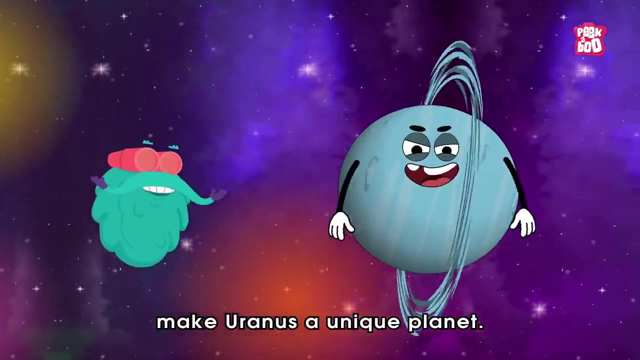 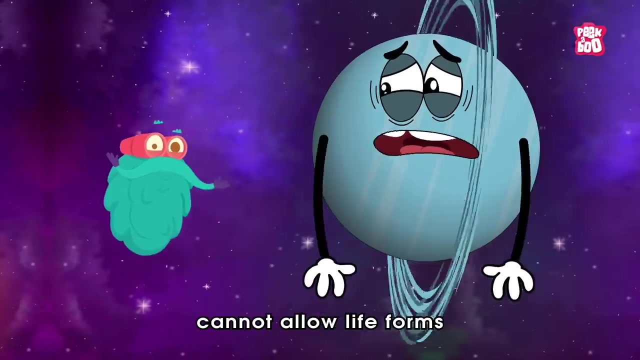 Not only that, but unlike the rings of other planets, which tend to spin horizontally, Uranus' rings spin vertically, like a Ferris wheel. All these features make Uranus a unique planet, But unfortunately, the same characteristics cannot allow lifeforms to survive on this planet.